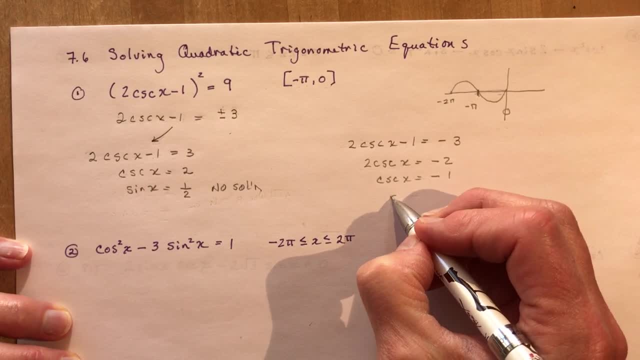 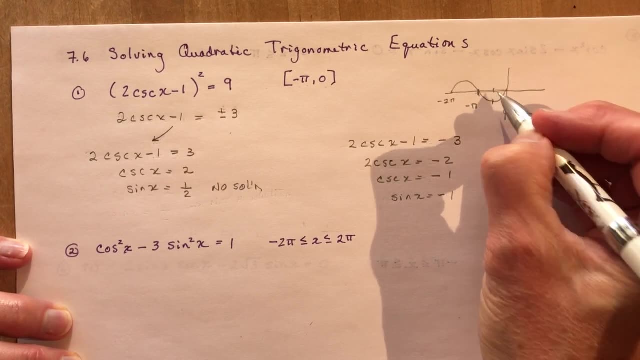 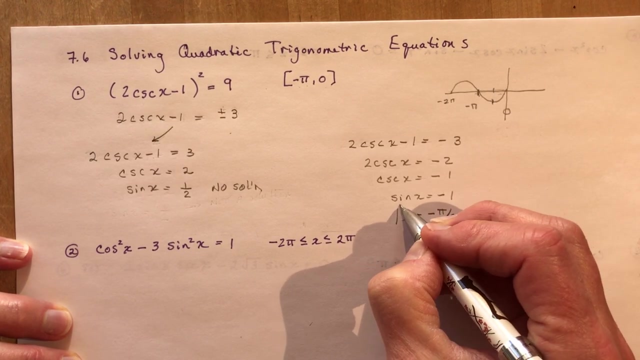 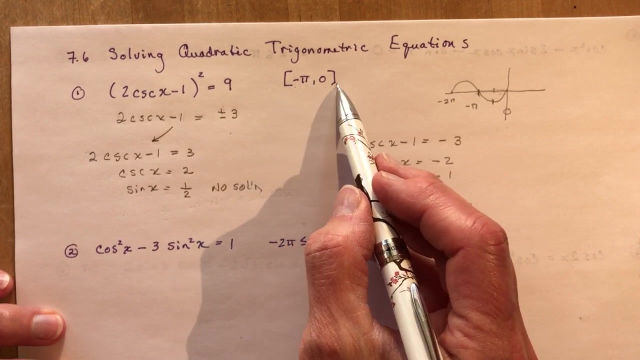 is equal to minus 1 or sine x equals minus 1.. And you can see by the graph here there's only going to be one solution, and that would be at x equals minus pi over 2.. So that's your only solution, And remember that we're looking at this interval here between minus pi and 0.. Okay, so the second. 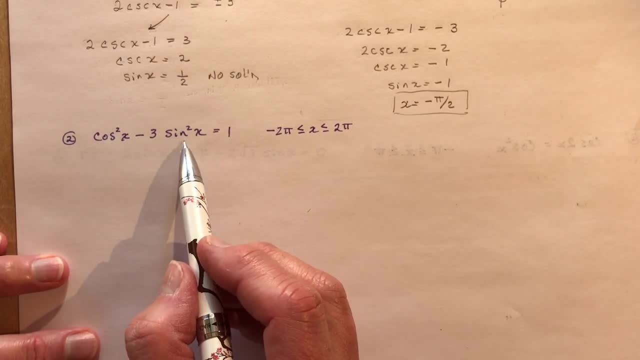 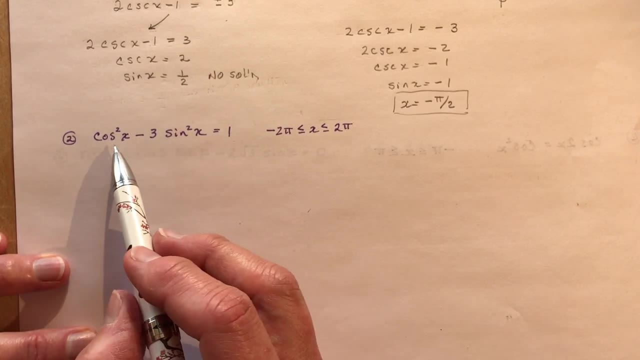 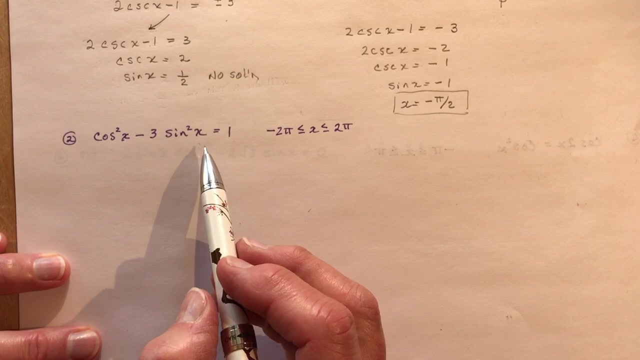 equation, we have cosecant x minus 3. sine squared x is equal to 1.. Now it's impossible to solve. This is like having an x squared and a y squared in an equation and trying to solve a quadratic. Okay, so the first thing you want to do is replace one of these, and it will work. 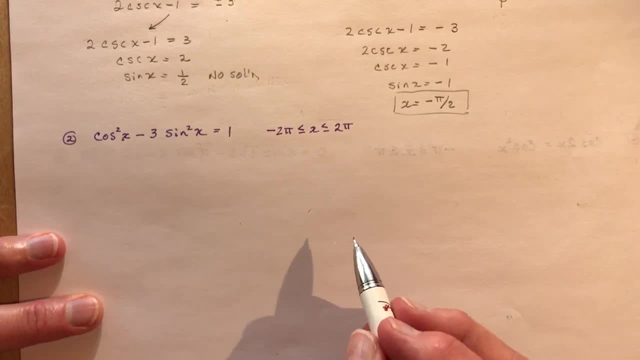 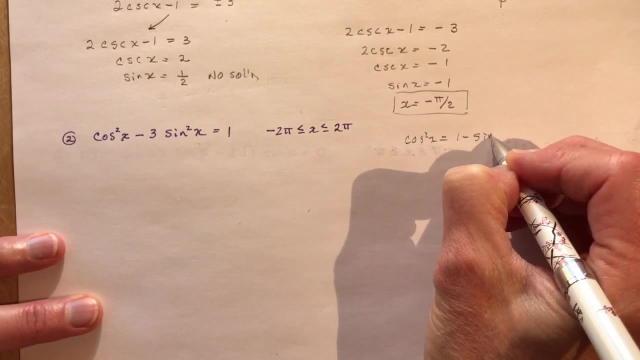 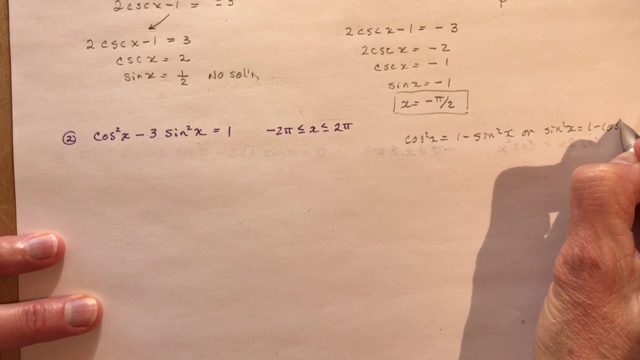 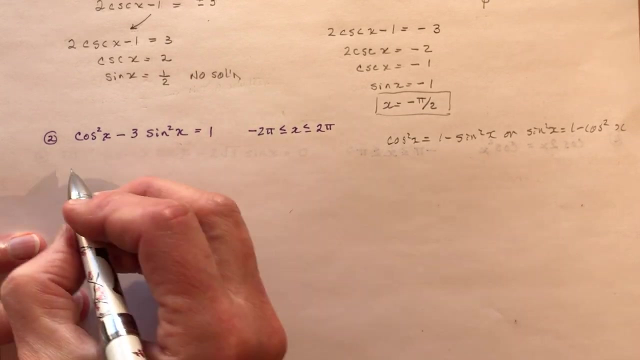 with either choice that you make. So I can say that cosecant x equals cosecant x equals 1 minus sine squared x, or I could do sine squared x equals 1 minus cosecant x. Okay, so you have the choice of which one you want to pick. I'll try the first one here. So I have 1 minus sine squared x. 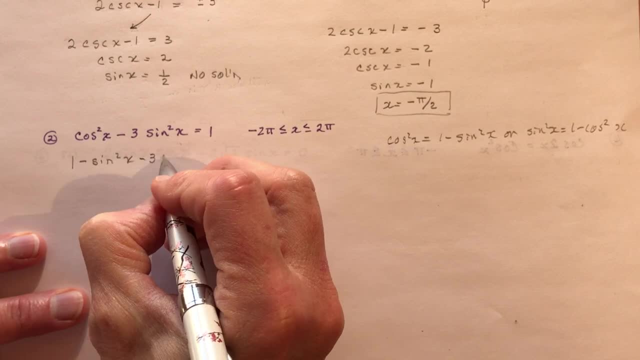 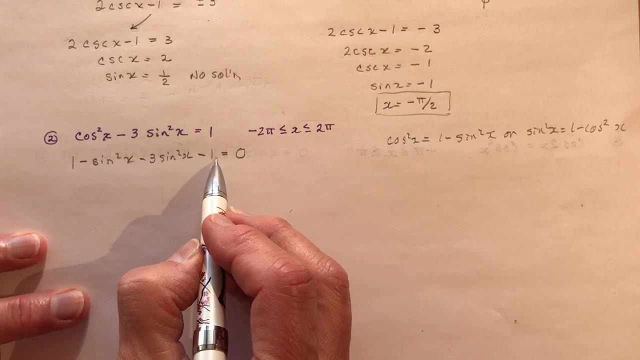 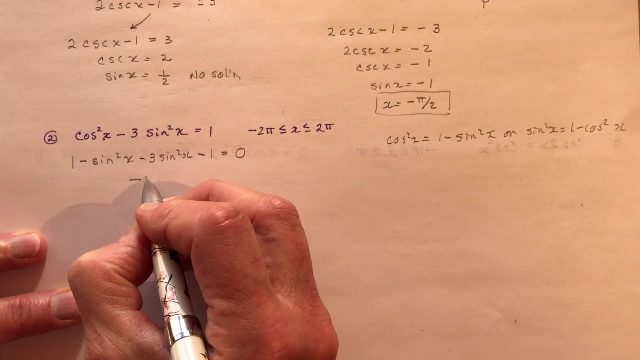 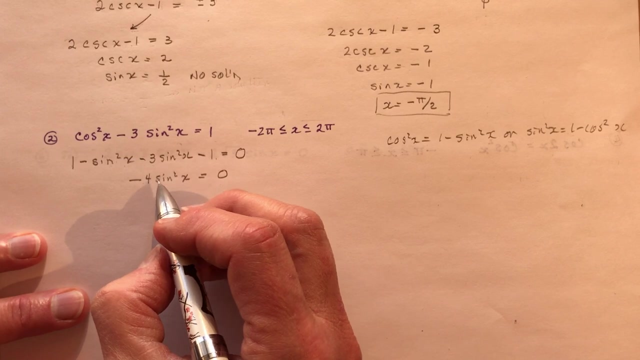 minus 3 sine squared x minus 1 is equal to 0.. So 1 minus 1, that's gone, and minus 2 sine squared x. minus 3 sine squared x, that would be minus 4 sine squared x, is equal to 0.. And you can see that if I 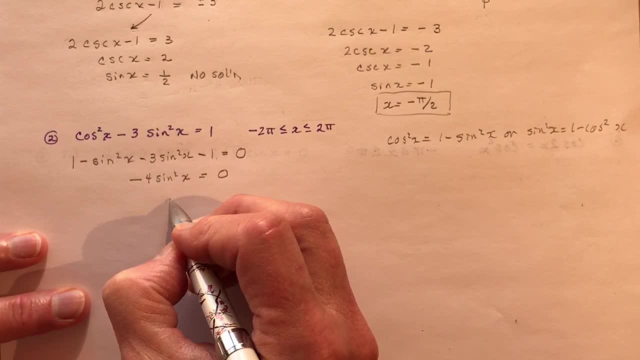 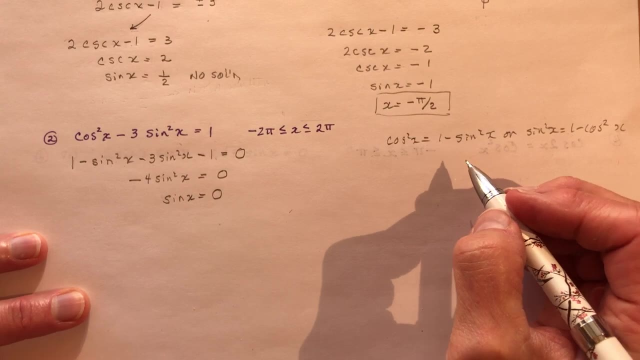 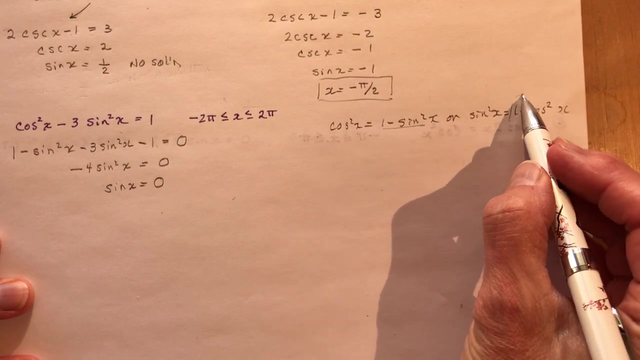 simplify that, I'm just going to end up with. sine x equals 0. So let's take a look at this one as well, using another equation. Instead of using this, we'll use 1 minus cosecant x and I'll show you how it still works. 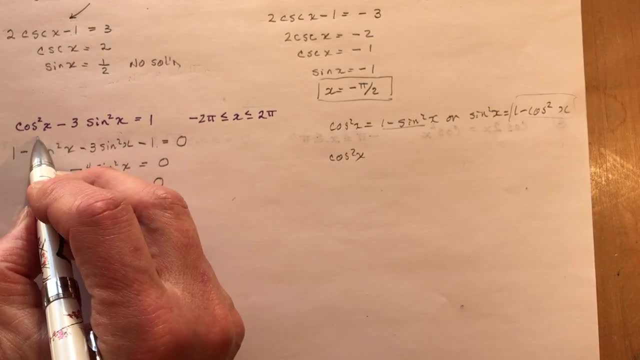 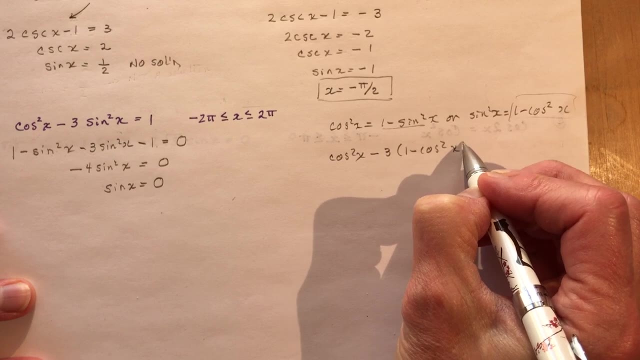 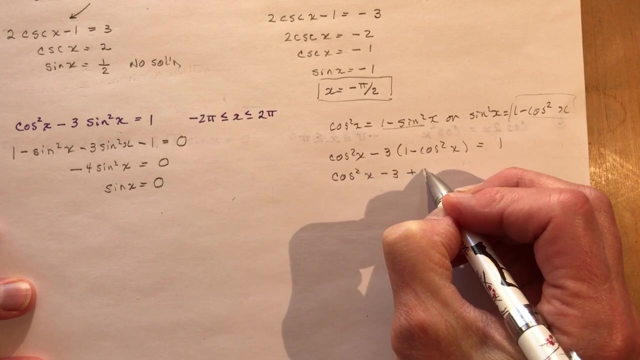 So I have cosecant x. I'm just coming back to over here. cosecant x minus 3 times 1 minus cosecant x is equal to 1.. So cosecant x minus 3 plus 3, cosecant x minus 1 is equal to 0.. 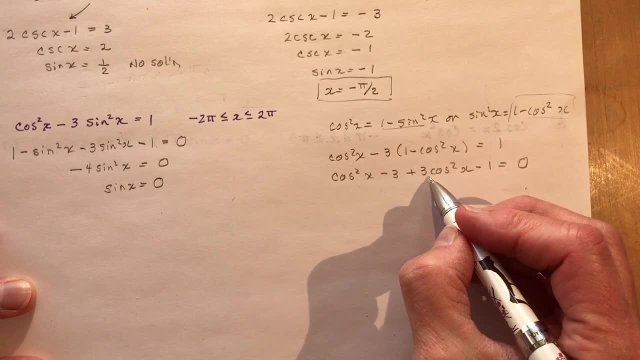 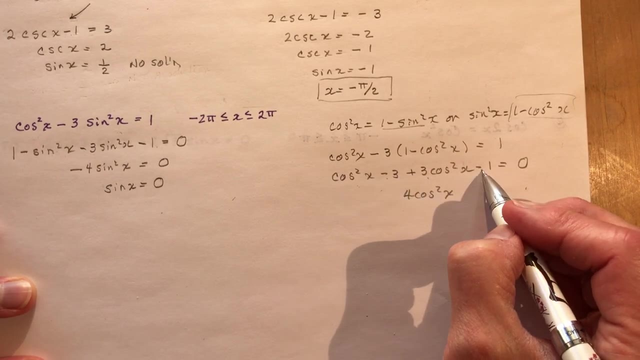 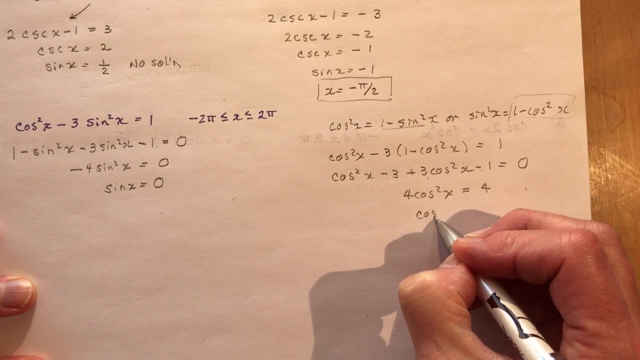 So now I have cosecant x plus 3. cosecant x, that's 4. cosecant x minus 3 minus 1. more is minus 4.. Bring it to the other side, Could have left that 1 there, I guess. So I get cosecant x. 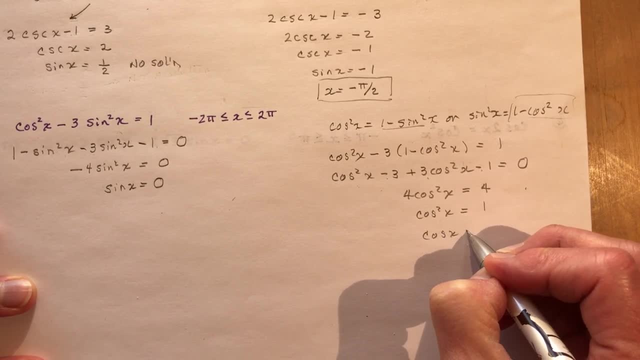 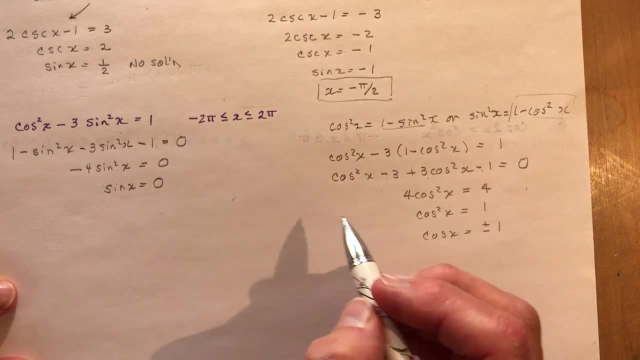 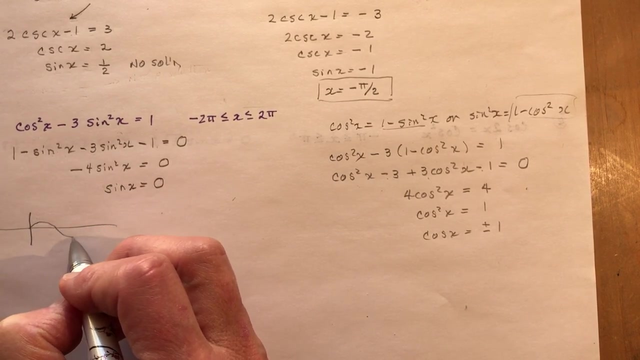 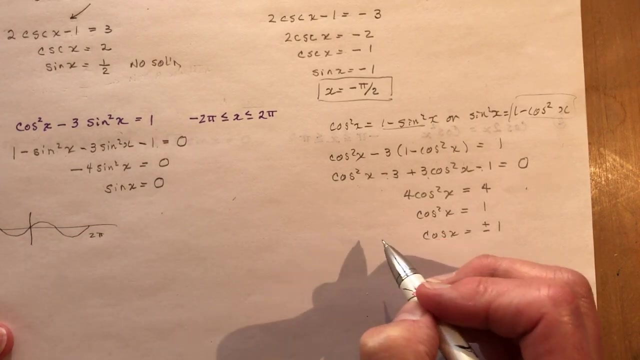 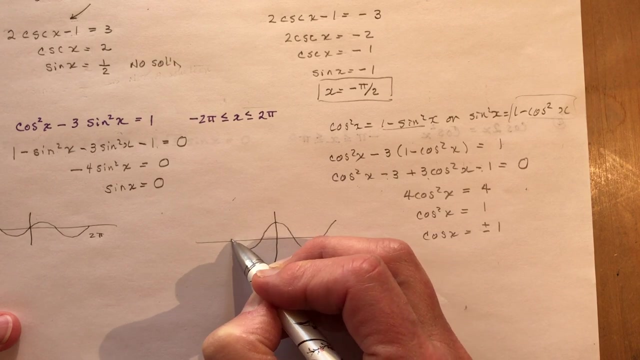 is equal to 1 and cosecant x is equal to plus or minus 1.. 2 pi and 2 pi. So for the sine function that would give me something like this: Here's minus 2 pi to 2 pi, And my cos function is going to go like this and like this. So there's my 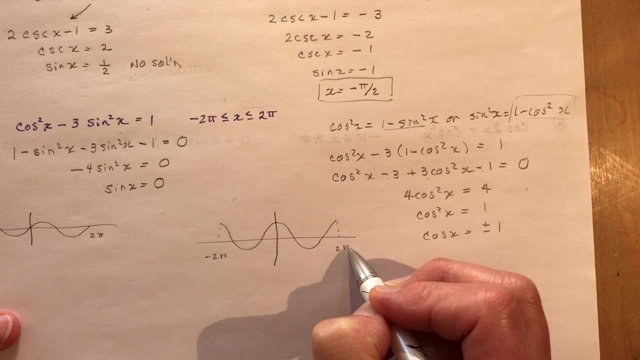 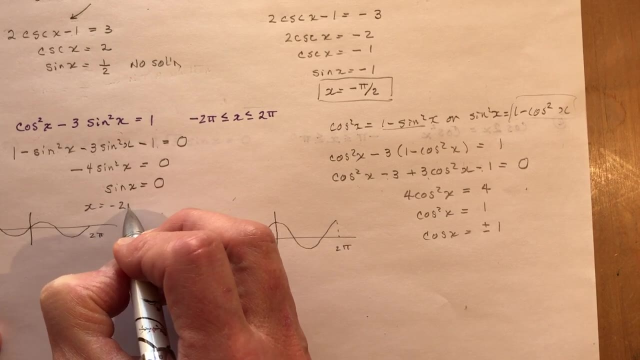 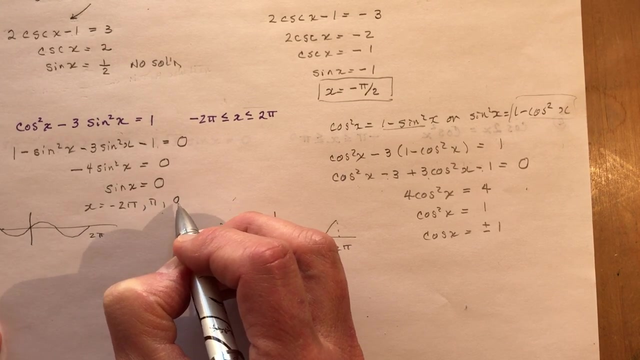 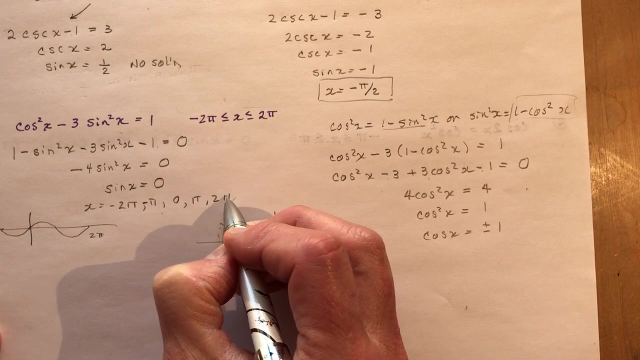 negative: 2 pi to 2 pi. So where's sine x equal to 0?? So we have minus 2 pi, Minus 2 pi. that's here This is going to be pi, then 0. I'm sorry, I forgot minus pi, 0 pi and 2 pi. And if we go to this equation here, 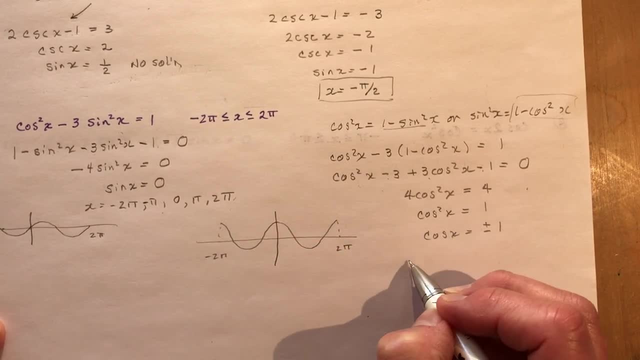 where's cos x equal to 1?? You'll see, I get x equals minus 2 pi. So plus or minus 1.. So that's this one, That's minus pi, And I think you can see that we're going to have the very same solution. 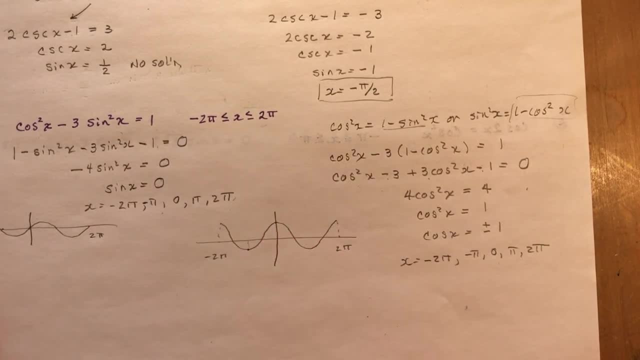 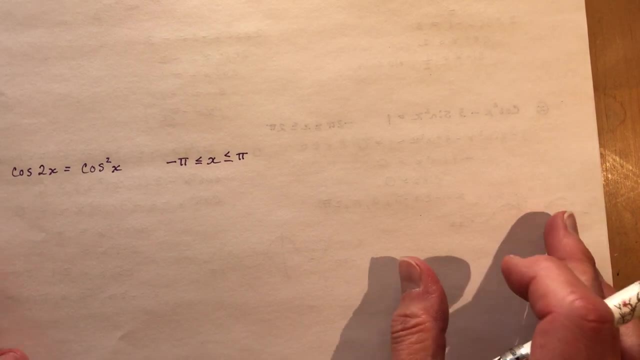 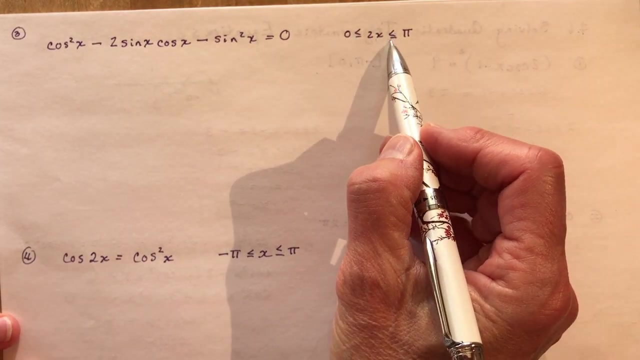 So it doesn't matter which one you choose, Just make sure that you're following the domain. Okay, flip the page Number 3.. cos squared x minus 2 sine x. cos x minus sine squared x equals 0.. 0 is less than or equal to 2x is less than or equal to pi. So you should simplify this first. 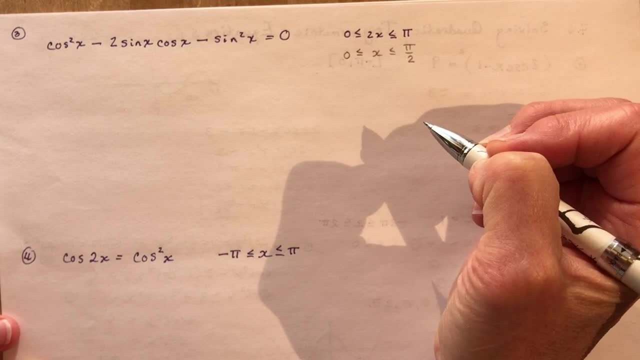 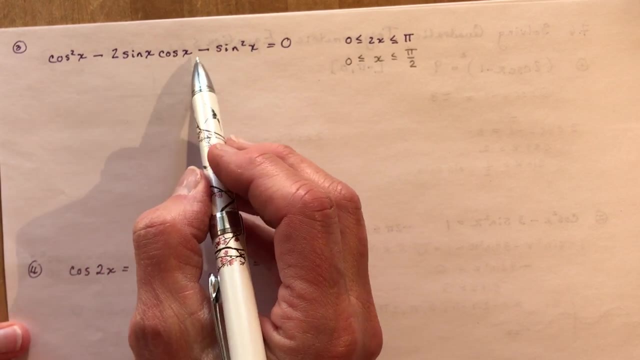 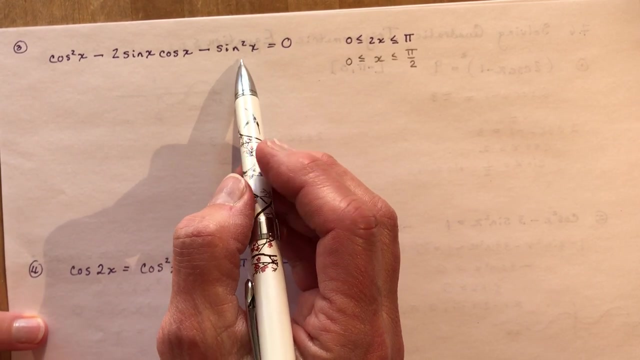 Divide everything by 2.. Okay, so that's the domain I want to use. This is my equation. Now, if you look at this equation, you'll see that there's no way you can make this into just one function by getting rid of the sine squared or the cos squared. 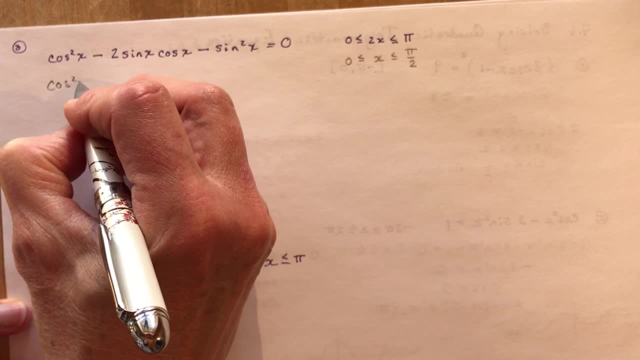 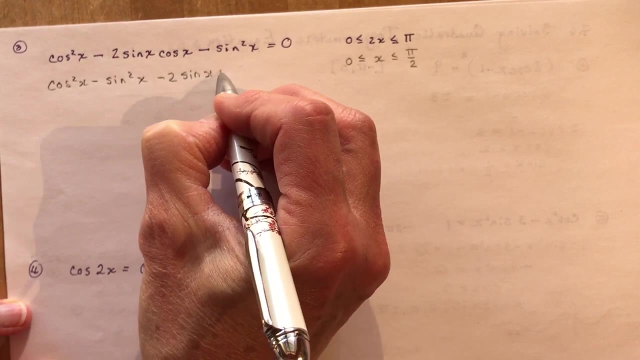 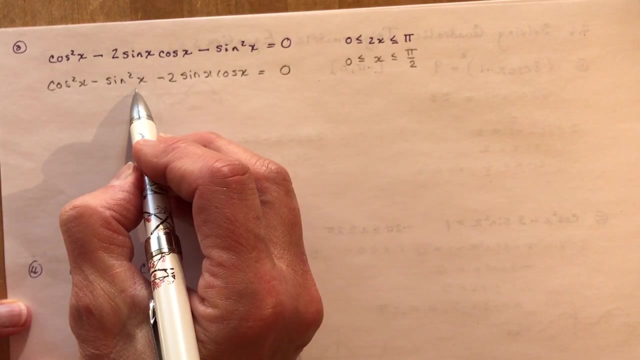 But if you look more carefully, or even sometimes, it's good enough for you to rearrange it to see what you might have here. Anytime you see 2 sine x, cos x, you should automatically be thinking of sine 2x. And what's this one cos squared x minus sine squared x. 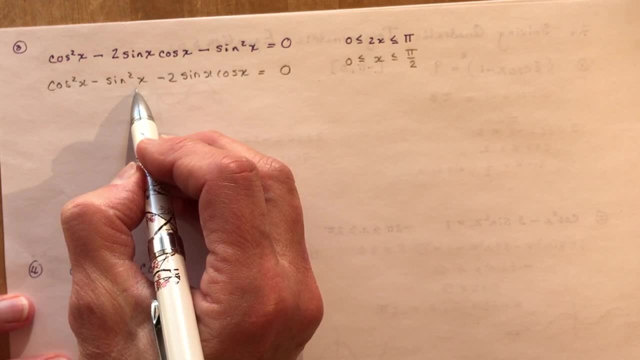 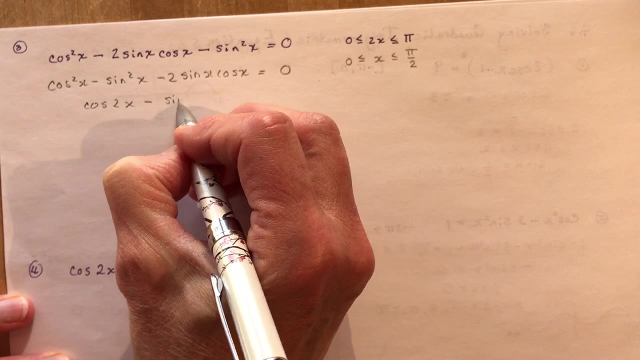 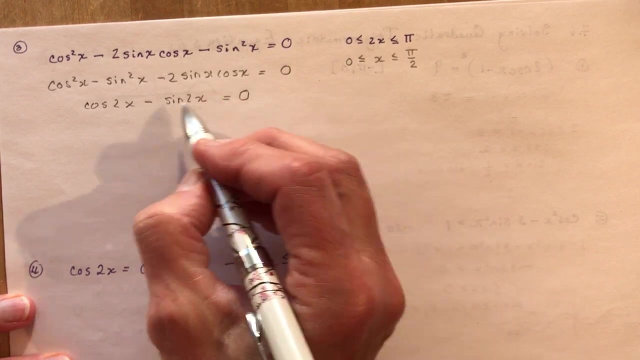 cos squared x minus sine squared x equals cos 2x. So we have cos 2x minus sine 2x is equal to 0.. Okay, so I'm going to have to make a fraction out of this, So I'm going to leave. 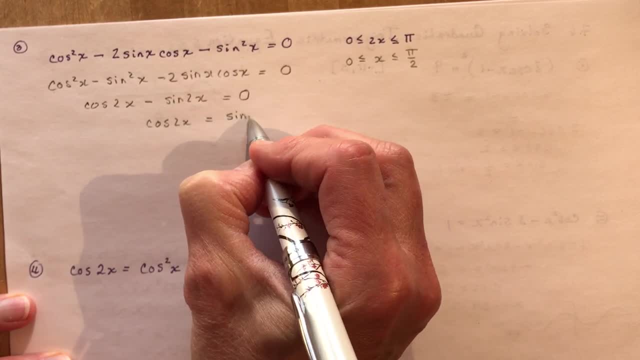 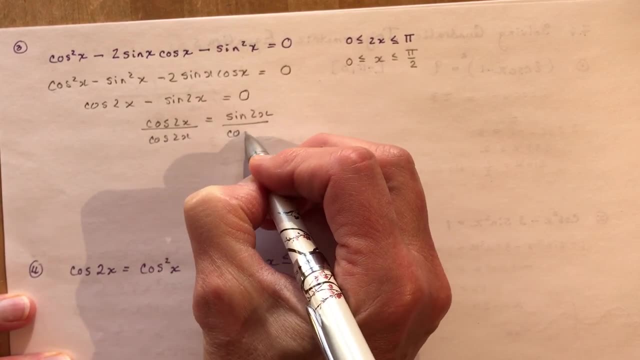 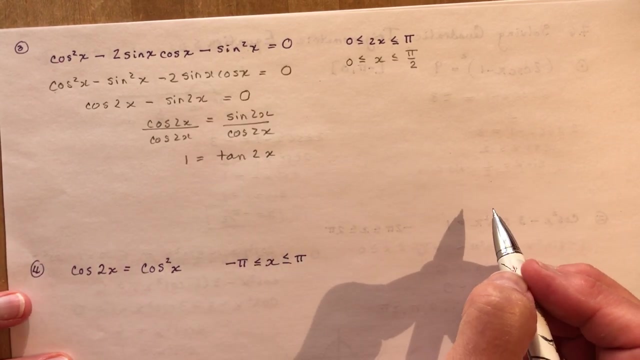 cos 2x here. Bring sine over here And I'm going to divide both sides by cos 2x And that's going to set me up for a nice solution of: 1 is equal to tan 2x, Okay, so where is tan x? 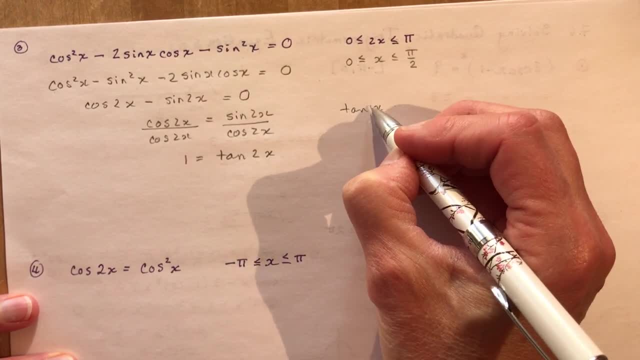 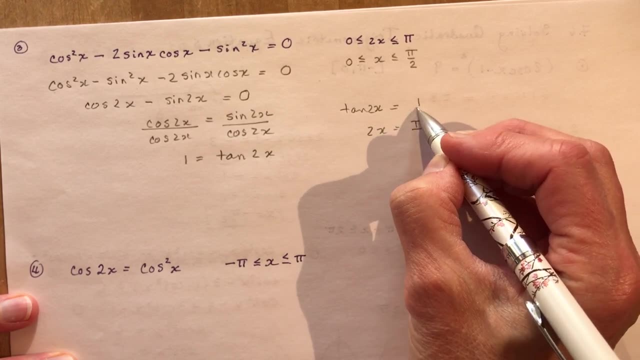 We've done one similar to this before. Where's tan 2x is equal to 1? So 2x is equal to pi over. where is this 1?? You know your special triangles by now: should be pi over 4.. 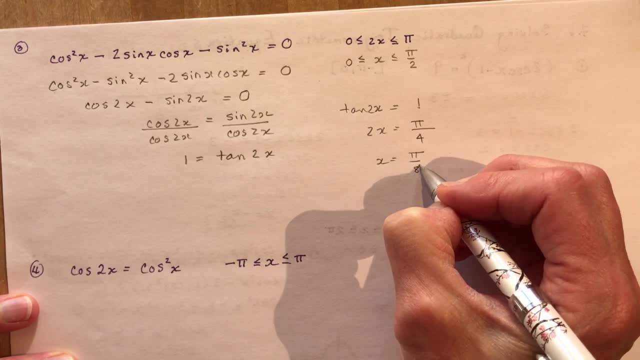 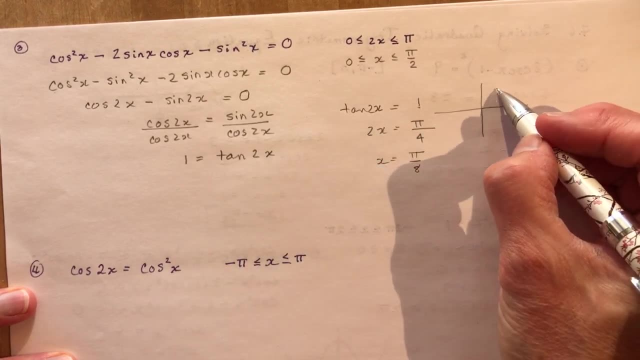 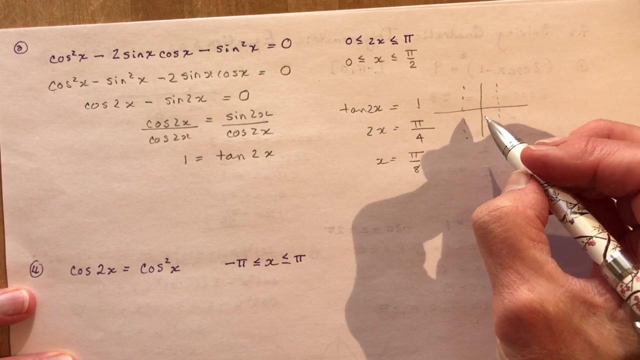 So that means x is equal to pi over 8. And if you sketched it, tan x, tan 2x has a period of pi over 2.. So that means this is going to be pi over 4.. We're between 0 and pi over 2. So it's going to be right here. 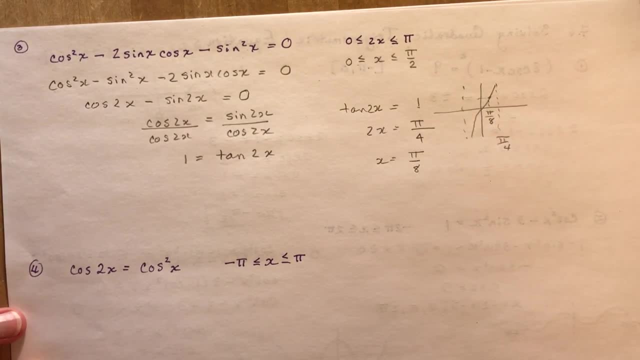 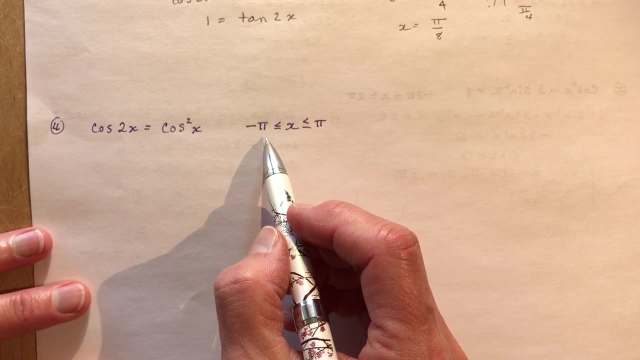 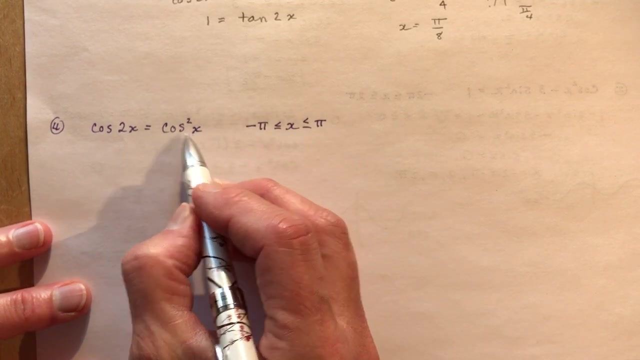 And that would be my pi over 8, just for a quick sketch for you. Okay, the next one: cos 2x equals cos squared x between minus pi and pi. So cos 2x and cos squared x, So I can replace this one. 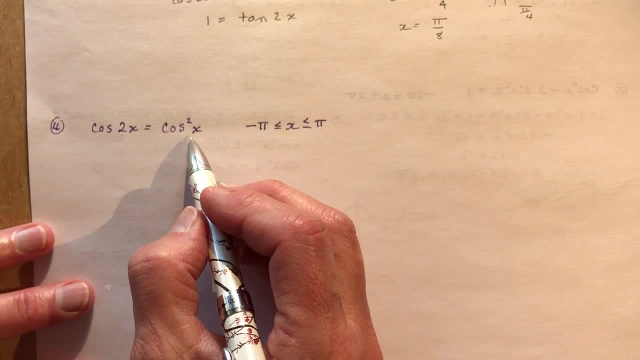 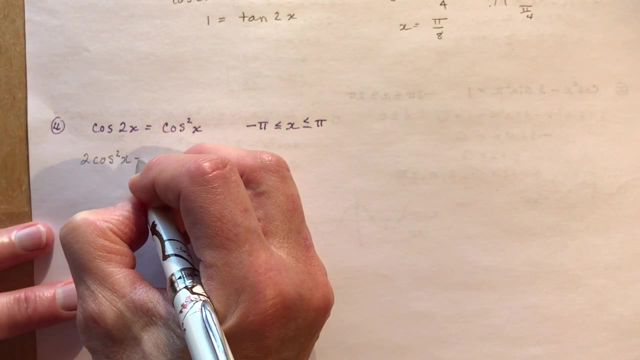 And if I want to keep everything in terms of cosine here, that will make things a little bit easier for me, right? So always look to find something: 2 cos squared x minus 1, that gives you just dealing with the same trigonometric function. 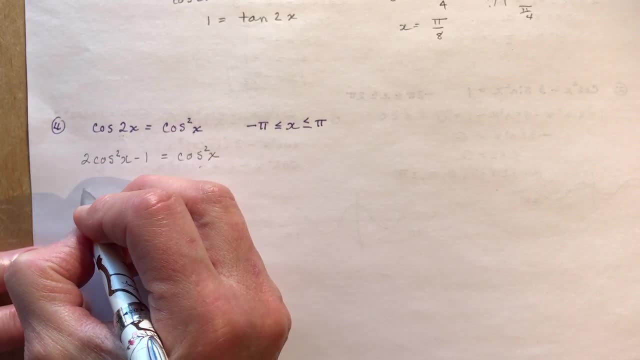 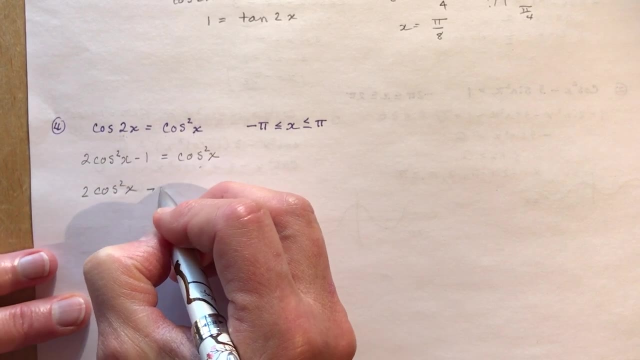 So now I'm going to rearrange, So I'm going to have 2 cos squared x minus a cos squared x. I'll write it on load. I already started the 2, minus cos squared x, And I'm going to bring the 1 over here. 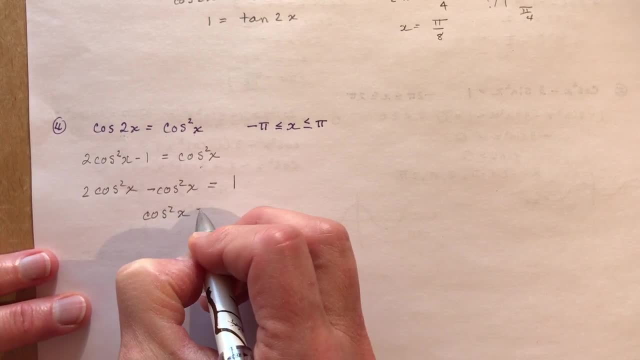 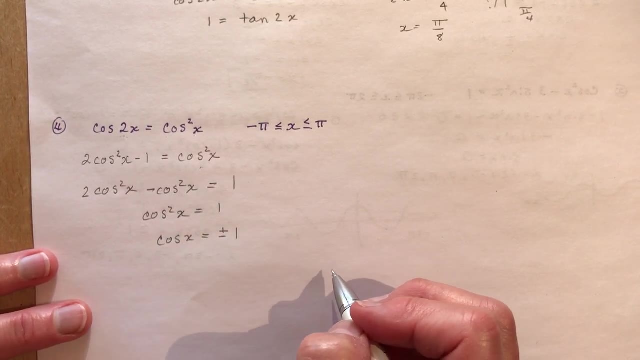 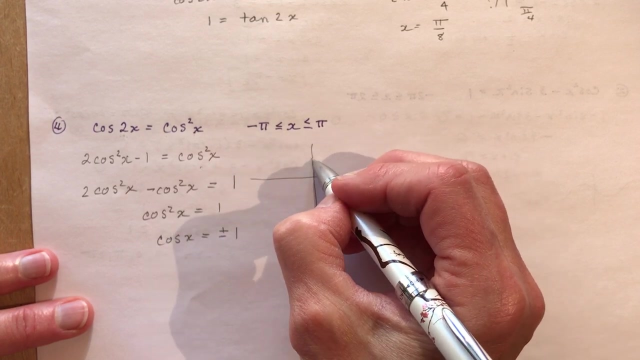 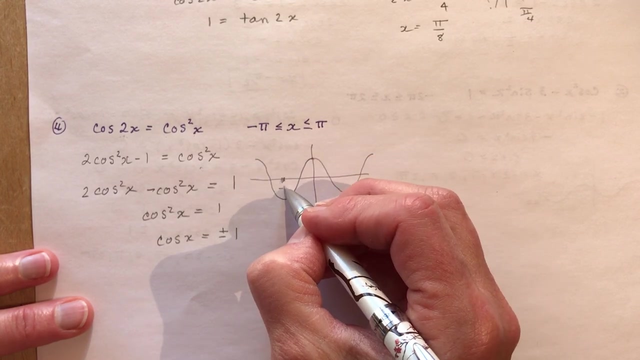 So now I have cos squared, x is equal to 1.. So cos x is equal to plus or minus 1.. So where is cos x equal to plus or minus 1?? And again you can make a quick sketch. So we're doing: this is cos and this is my minus pi and my pi. 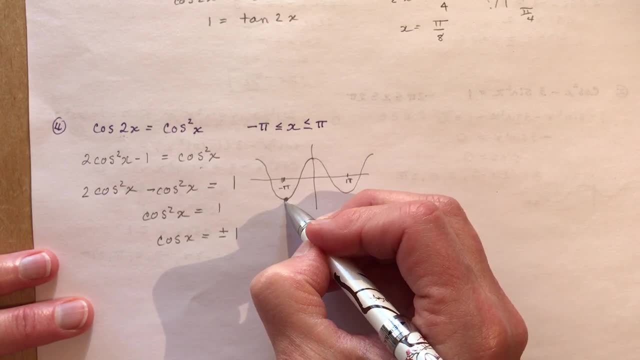 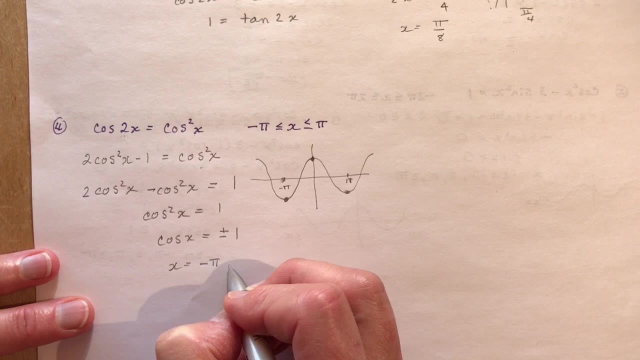 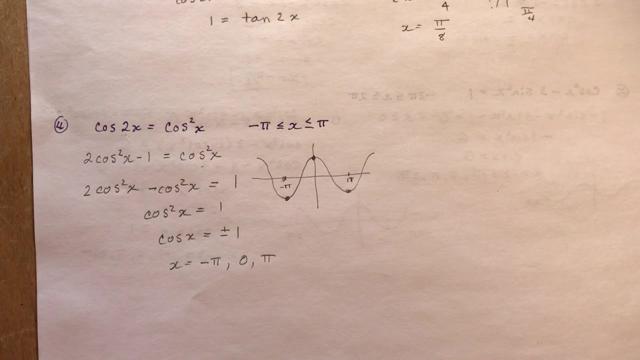 And where is it equal to plus or minus 1?? So we have this solution, this solution, and this solution. So x is equal to minus pi 0, and pi. Okay, so you could do the same thing, you could do another, do this another way if you, if you want to try it another way. 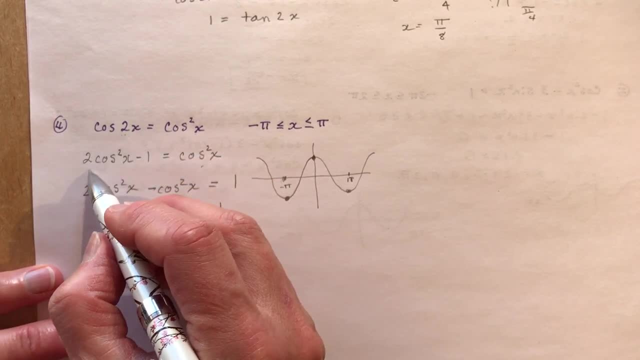 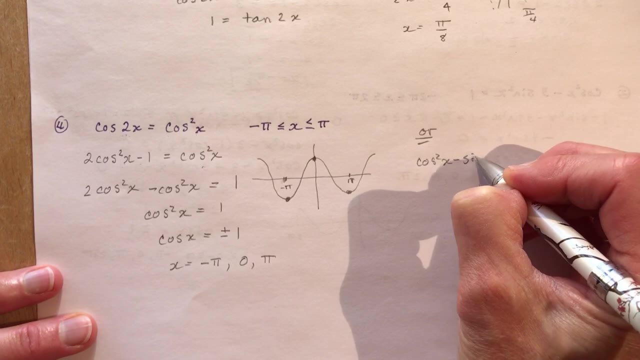 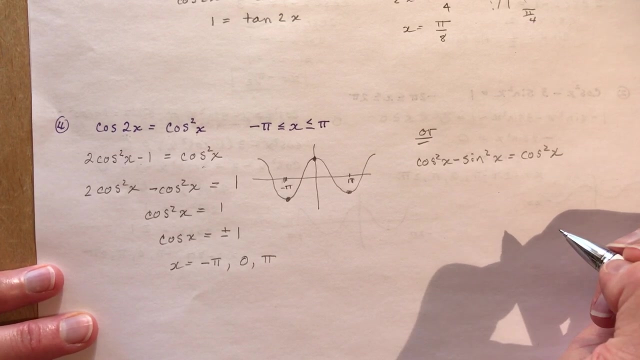 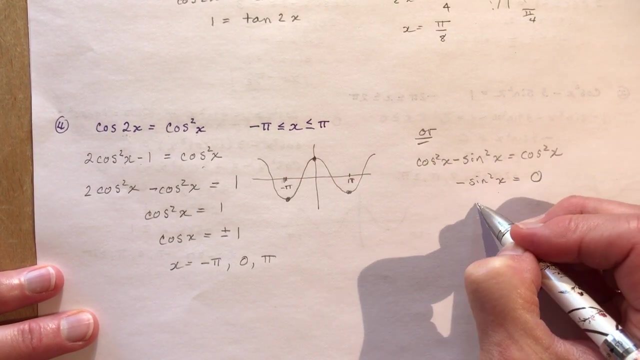 So we could use, instead of 2 cos squared x minus 1, we could have used cos squared x minus sine squared x equals cos squared x, And that obviously is going to give you minus sine squared x- maybe this one's easier. equal to 0, sine squared x equals 0, and sine x equals 0.. 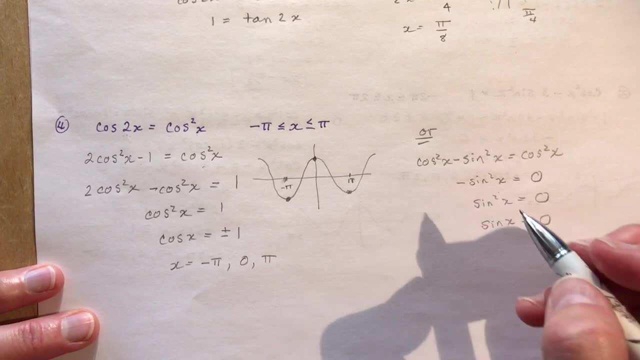 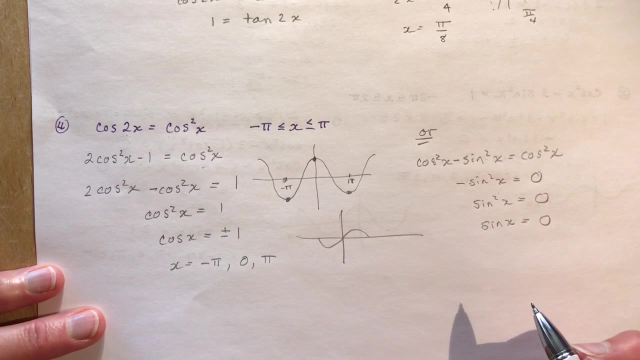 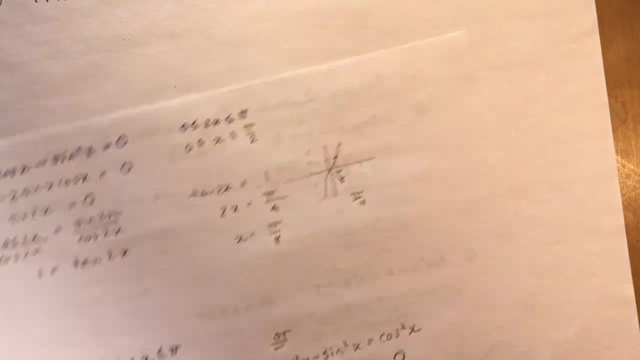 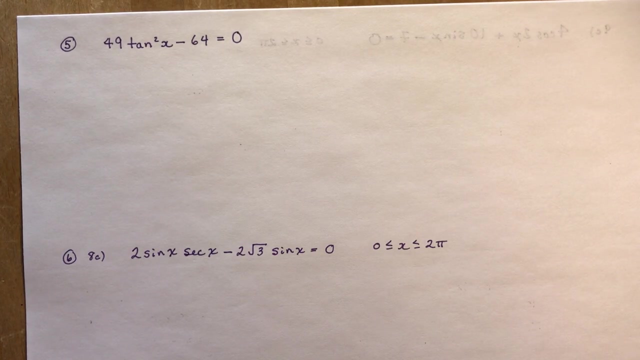 zero. so if you sketched the sine function now between minus pi and pi, you would end up where is it? zero. you end up with the very same solutions. okay, okay, number five. I've got- um well, I'm sure you can recognize what this is right away- 49 tan squared minus 64. that, of course, is a difference of squares. so 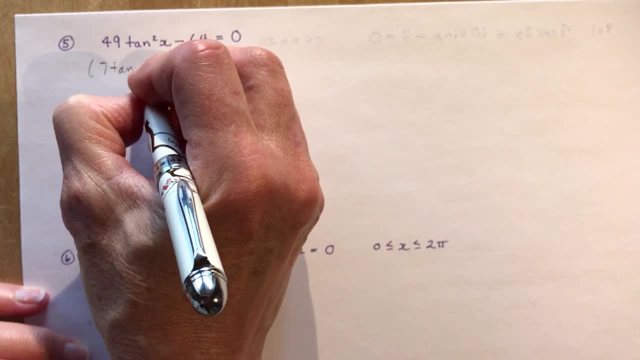 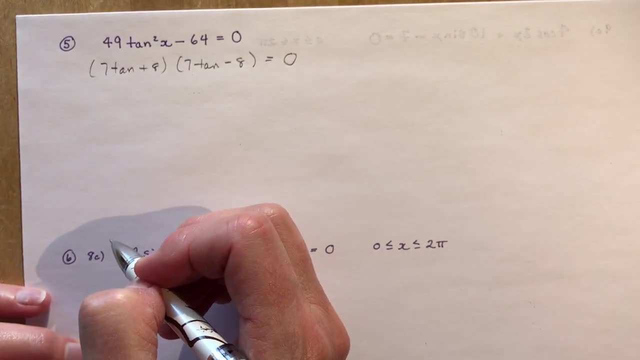 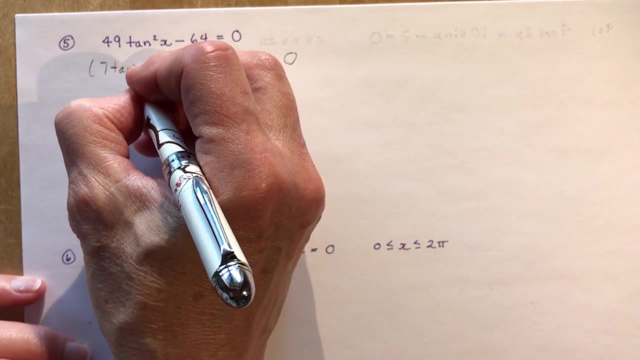 that's going to give you 7 tan plus 8 times 7 tan minus 8 equals 0. and then you have two equations to solve. I'm not going to finish this for you. I'm sure you can figure. I'm sorry. this should be 7 tan X. I have a cold. can you tell my 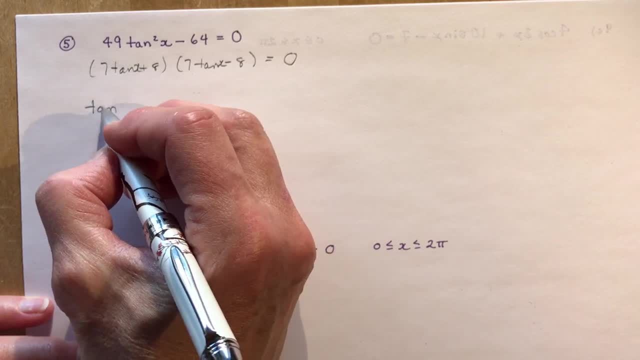 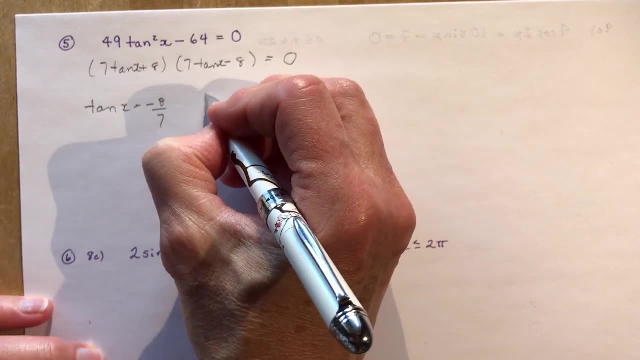 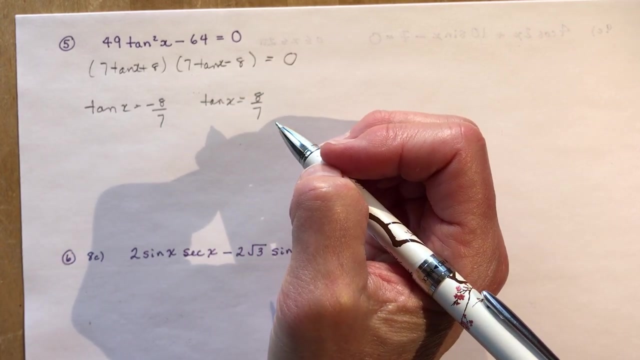 brain isn't working quite as well as it should be. so tan X equals: bring the silver. so B minus 8 over 7, and tan X equals 8 over 7. okay, so now all you're going to do is use your calculator and find I didn't give a domain for this one. I 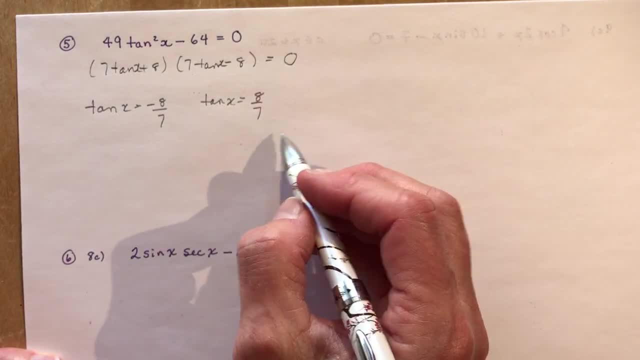 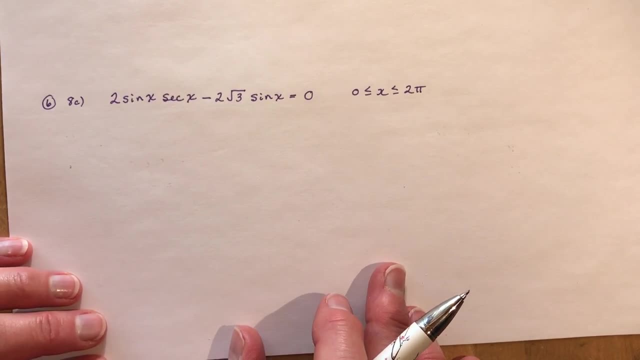 think it might be an example out of your textbook, one of your homework questions, so you can check that out. okay, this is also a question from your homework or your textbook, I'm sorry. 8c it says 2 sin x secant x minus 2. 3rd sin x equals. 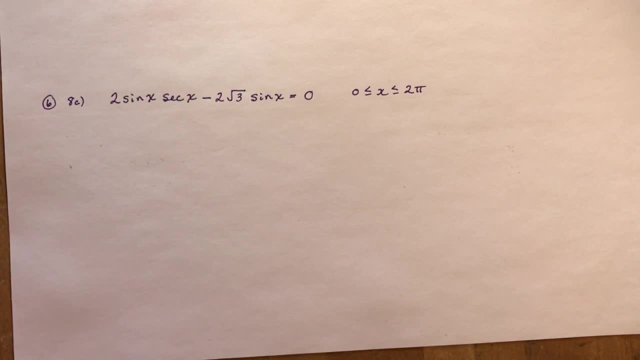 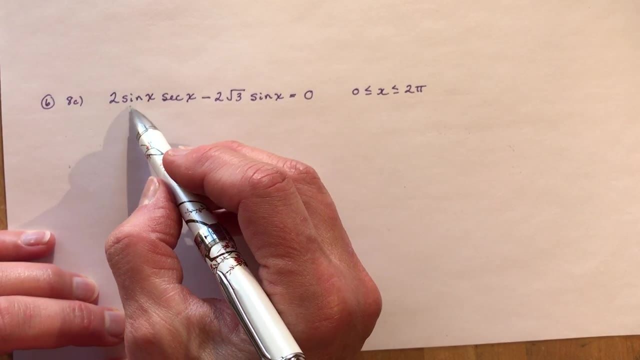 0. so I chose this one for a demonstration because it it requires you to do some factoring. so if you said: well, what can I do? I could write: this is 1 over cos, and then you're not getting anywhere, right, you'd have sine over cos. 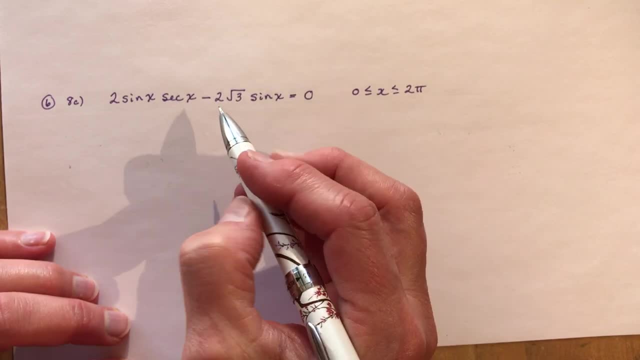 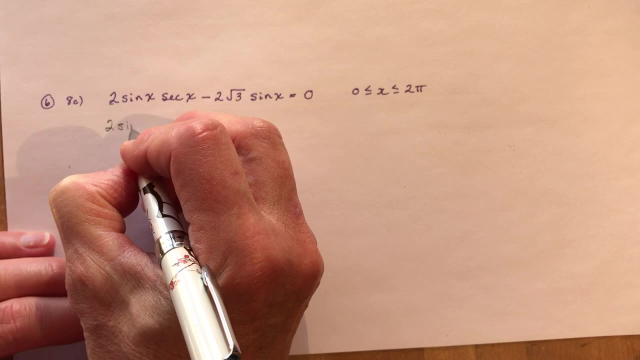 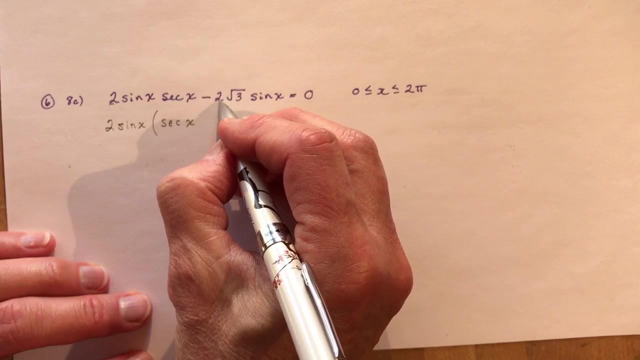 it's tan and you still have a sign and no. so you have to just kind of be a little creative here. so if I take out a 2 and a sin x, I think you'll see that I could have secant x and take out this 2 and a sin x and I get minus root 3. 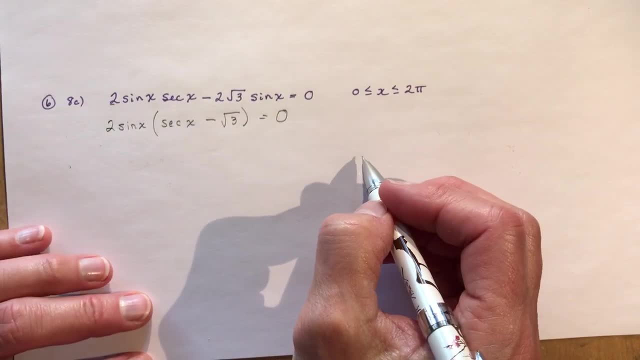 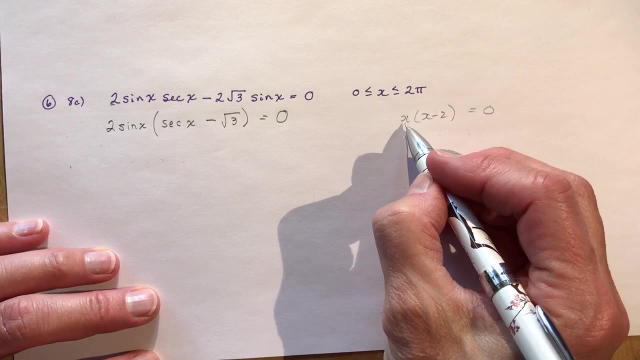 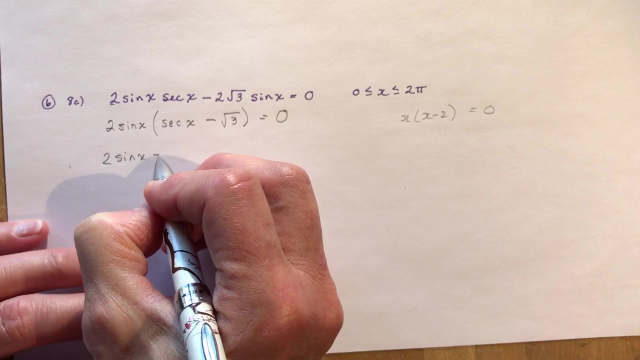 equals 0. so what are the two solutions? would be like me saying: oh, I have x, and x minus 2 equals zero. what's x equal to? You say: well, this is zero or this part's zero. So the same thing here. So I have: where is two sine x equal to zero And where is secant x minus root three? 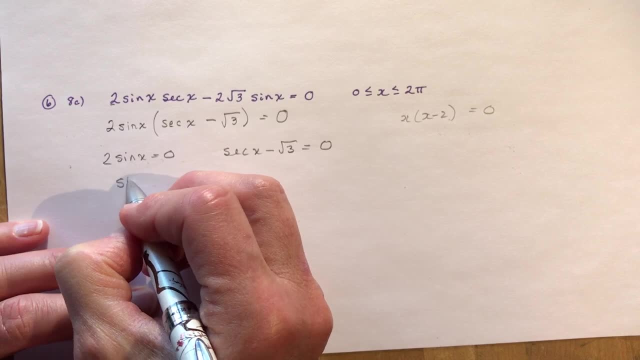 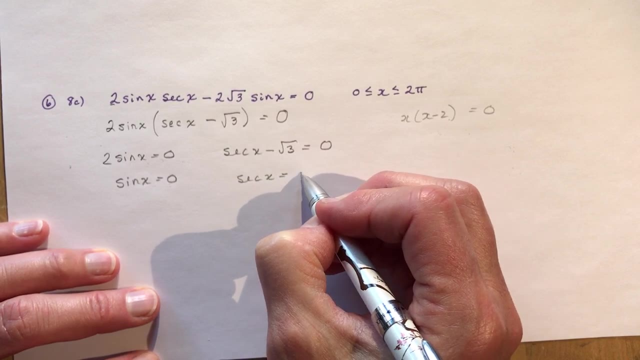 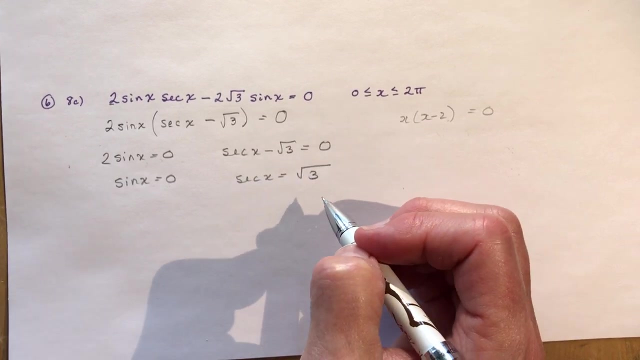 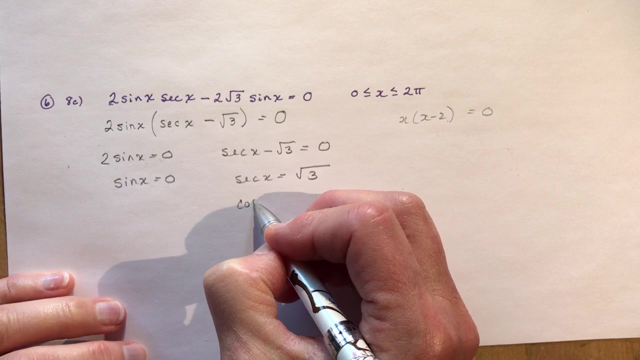 equal zero. So that's just sine x equals zero And this is secant x equals zero. Oh, no, sorry, root three. What am I saying? Secant x equals root three. Now, root three, that's not a special triangle solution. So if I said cos x equals one over root three, 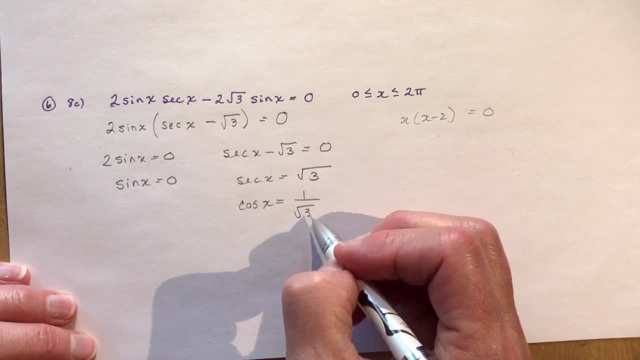 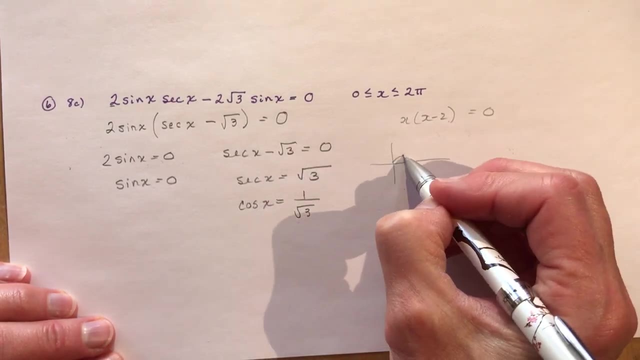 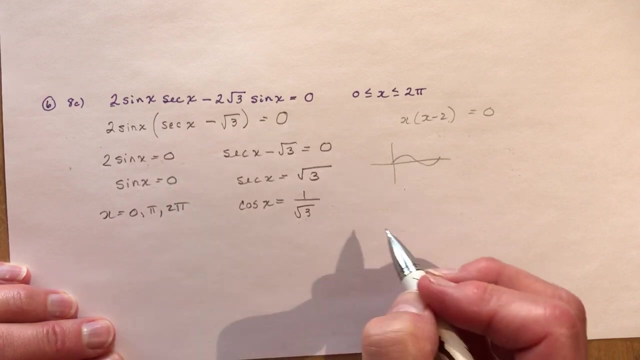 that would be the same, the same equation, right? So where sine x equal to zero, between zero and two pi. Oh, that's pretty easy: Zero and two pi. So zero pi, 2 pi, and for cos, x equals 1 over root 3. you could use your calculator for this, and I'm just. 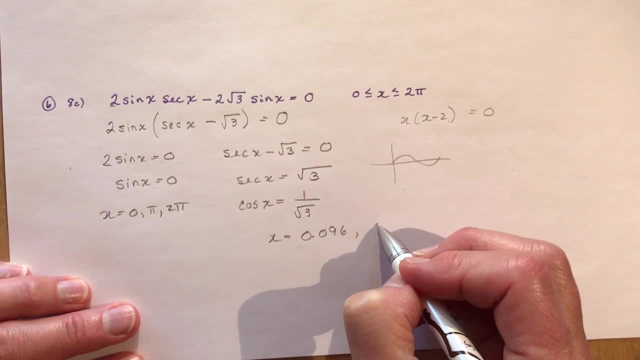 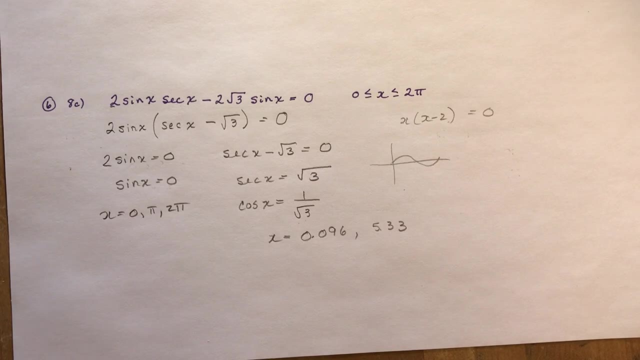 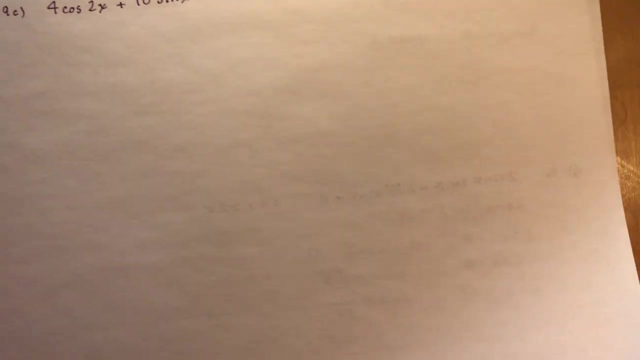 going to tell you what the answers are. and 5.33, so you make sure you're in the right quadrants, okay, so I have one more example to do for you, and this one requires a little more factoring. that's why I picked this one as well. so we have. this is 9c from your homework. it says for cos 2x: 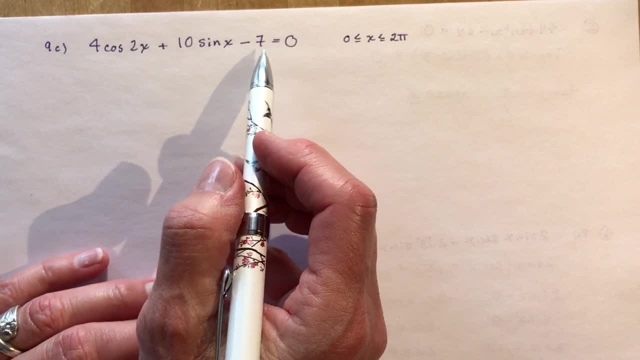 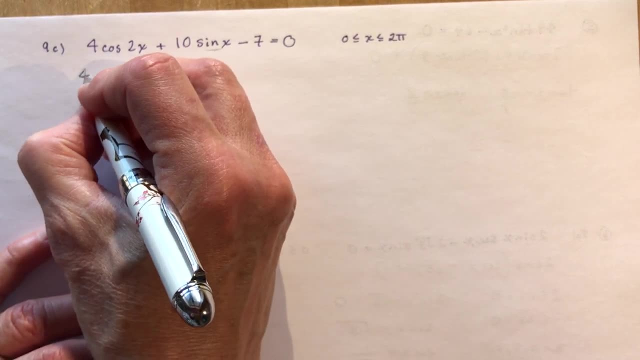 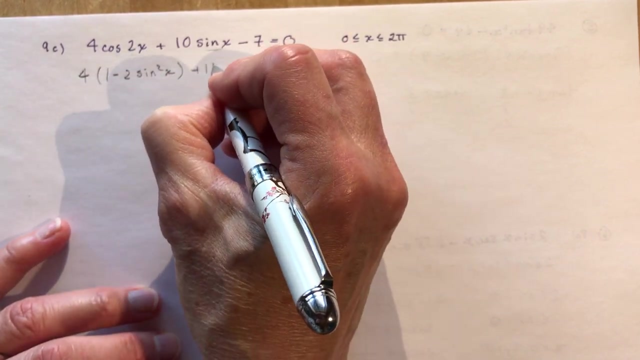 plus 10. sin x minus 7 equals 0, so I want to write it in terms of sin x, so cos 2x. we're going to replace cos 2x by 1 minus 2. sin squared x plus 10, sin x minus 7 equals 0. 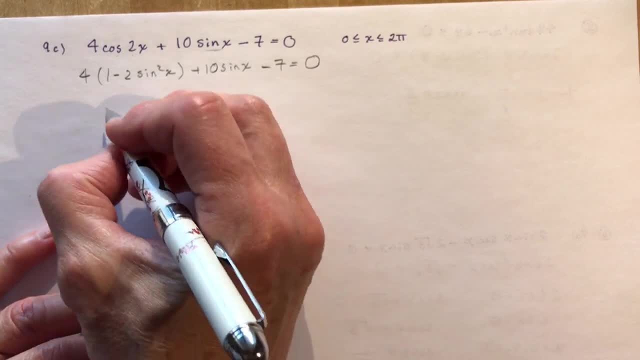 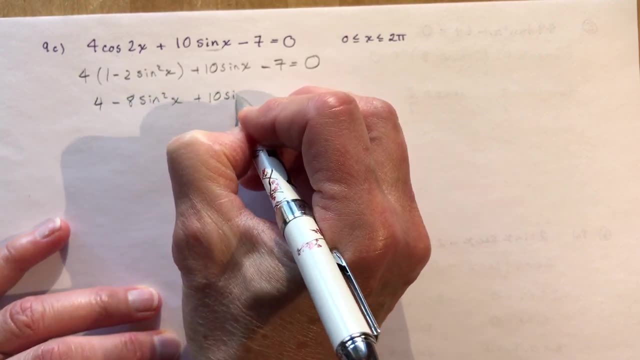 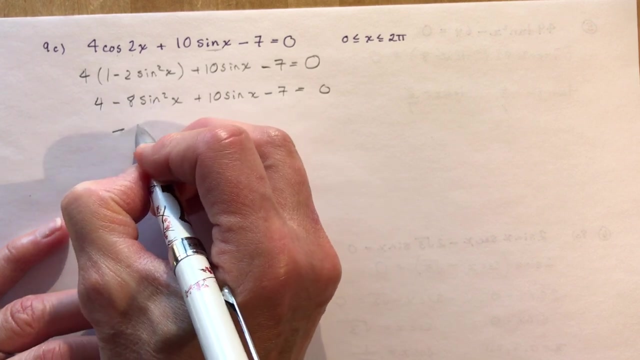 okay. so now I'm going to expand. so I had 4 minus 8 sin squared x plus 10 sin x minus 7 equals 0. I can combine just the two numbers, so I have 8 minus 8 sin squared x plus 10 sin x. 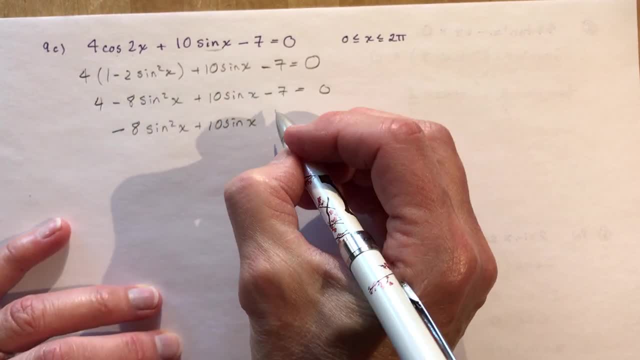 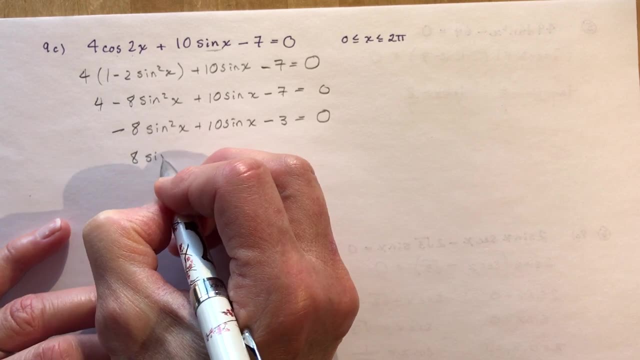 positive. 4 minus 7, that would be minus 3, equals 0 and remember, I'm going to expand. so I have 4 minus 8, sin squared x plus 10. sin x plus 10, sin x multiplies it by 8 minus 7.5, and now I have 8 minus 8, sin squared y minus 3, x minus. 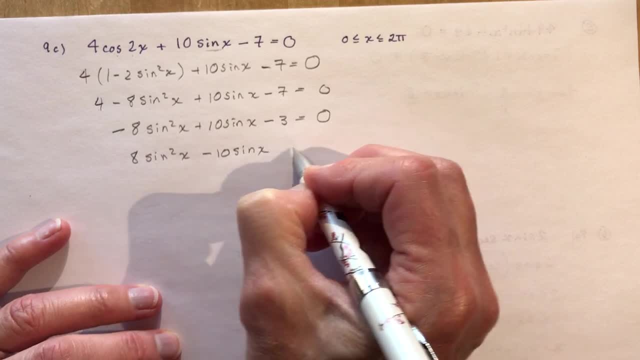 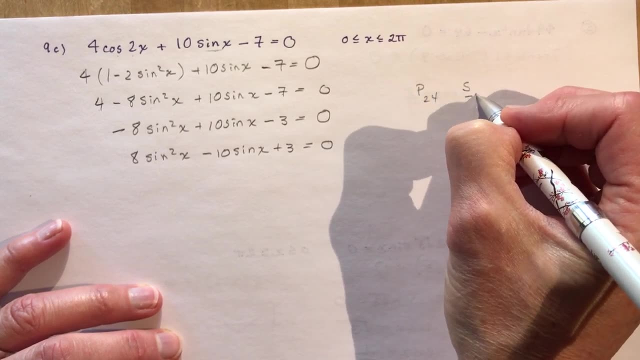 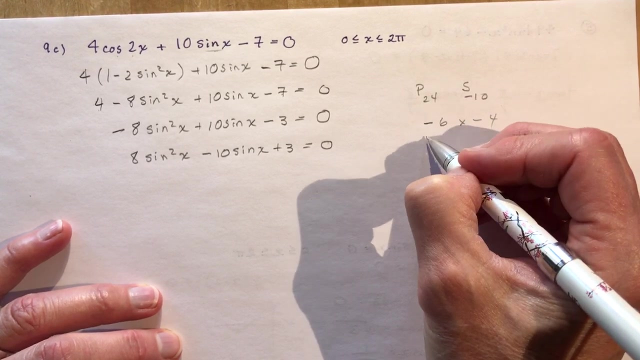 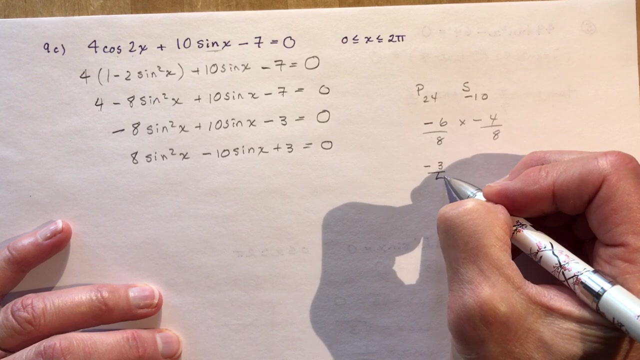 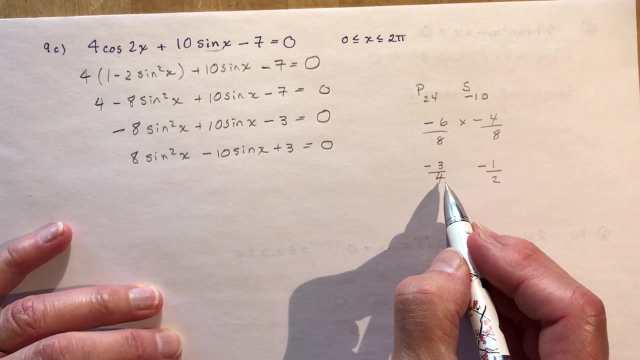 30, which then I have 8 minus 8. sin squared x plus 1, x minus 1 is equal to m, And this is going to be minus 1 over 2. So that gives me 4.. Now, remember, this is just like sine squared x. 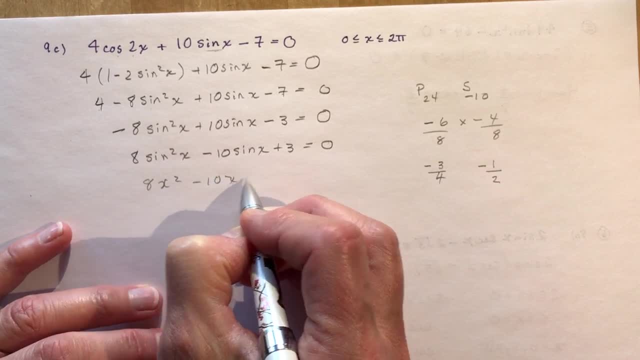 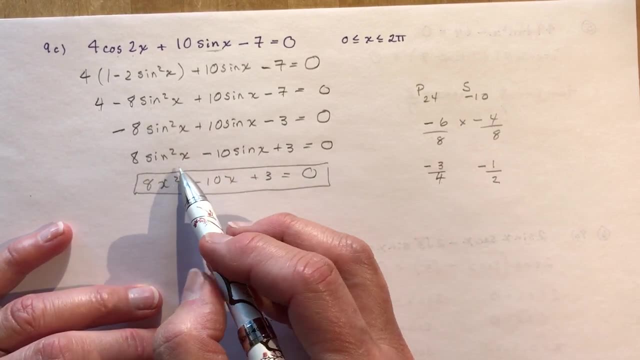 I could have written this like this: 8x squared minus 10x plus 3. And you would know how to factor this right. So, if you need to, you can say: let sine x equal x and then write out your equation. 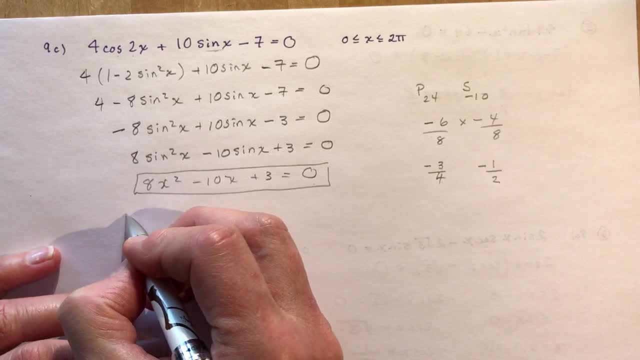 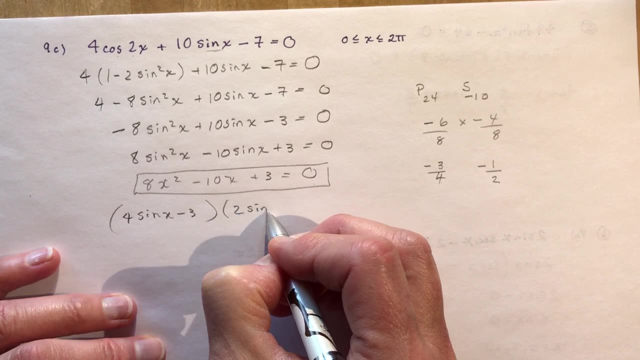 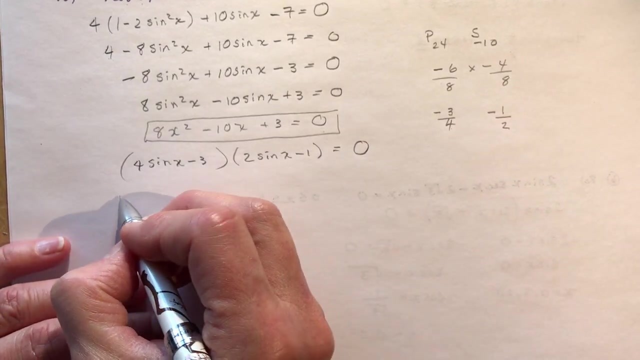 and then just substitute it back in in the end. So I get 4 sine x minus 3 times 2. sine x minus 1 is equal to 0. And now I solve each of these little bracketed forms So I would get sine x equals 3 quarters, which isn't a special triangle. 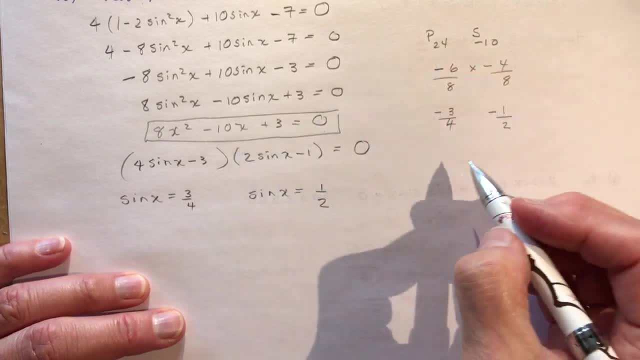 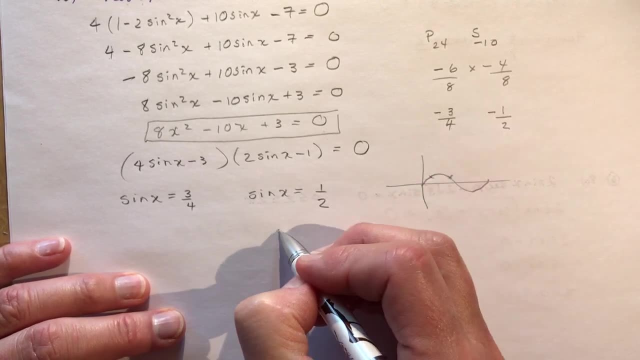 and sine x equals 1 half And I'm between 0 and 2 pi. So 0 to 2 pi, That means sine x is a half. We know those. That's x equals pi over 6 and 5 pi over 6.. 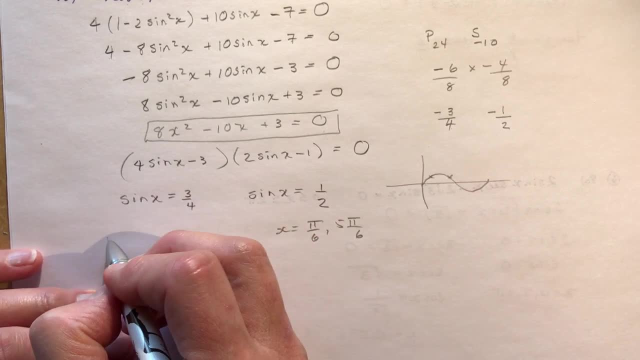 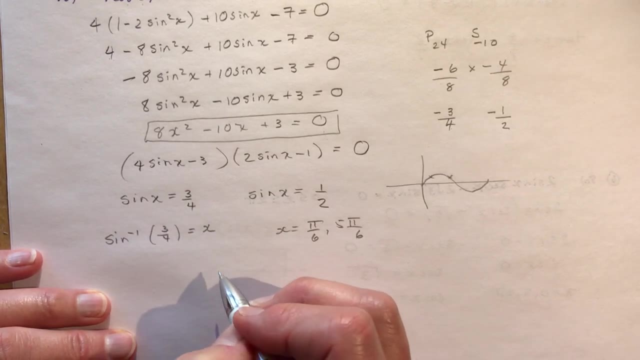 And sine x equals 3 quarters. Well, you're going to have to do some calculator work. That's going to give you your x value And that's going to give you, let me see, 0.85.. That's 1.. 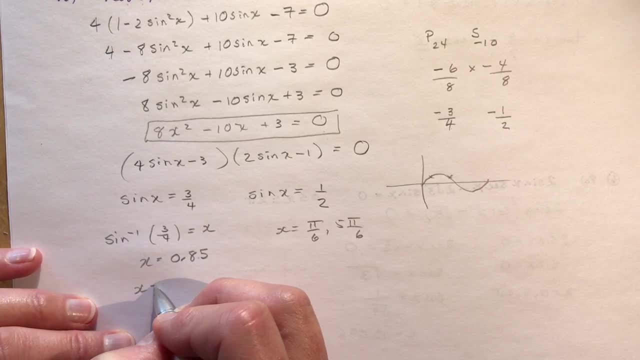 So that's in the first quadrant. In the second quadrant it would be x. So that equals 3.14 minus that And that's going to give you approximately 2.29.. Okay, so hopefully that helps straighten out some of the things you could do. 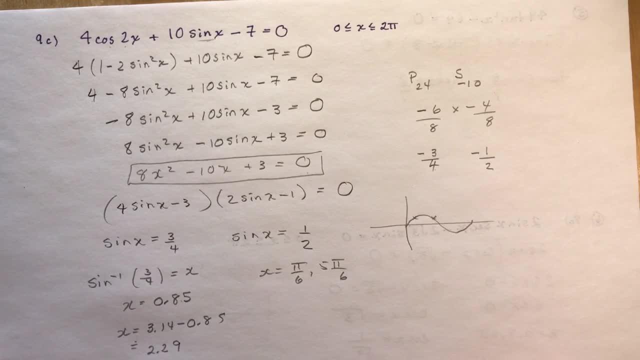 with quadratic trigonometric equations. Please give me a thumbs up if you enjoyed the video, And don't forget to subscribe and support the channel. I'll keep on working for you. Bye.